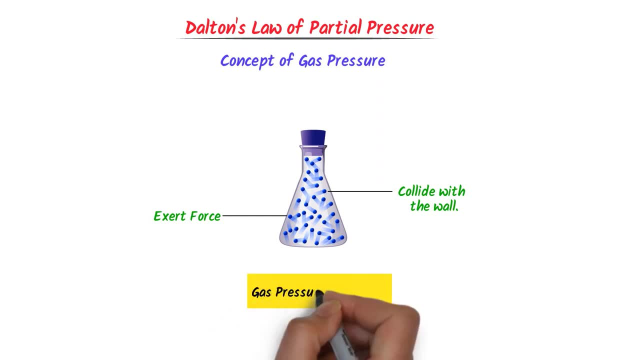 walls of the container. Or we say gas pressure is equal to force per unit area. Therefore we say that gas pressure means the particles constantly exert force on a unit area of the container. Let me repeat it: the particles constantly exert force on a unit area of the. 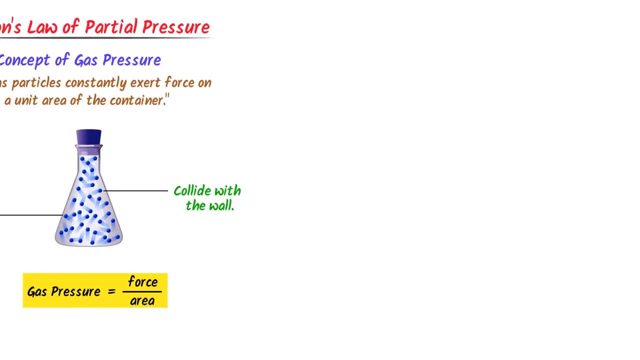 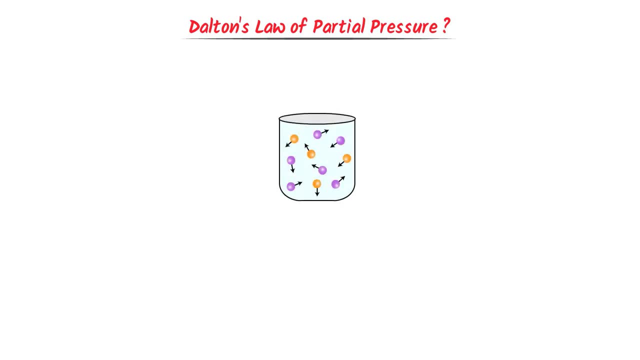 container. Hence noted down this basic concept. Now, what is Dalton's Law of Partial Pressure? Well, consider this container. It contains a mixture of non-reacting gases like hydrogen gas and oxygen gas gas. Remember that I use the word non-reacting gases. It means that hydrogen gas and oxygen. 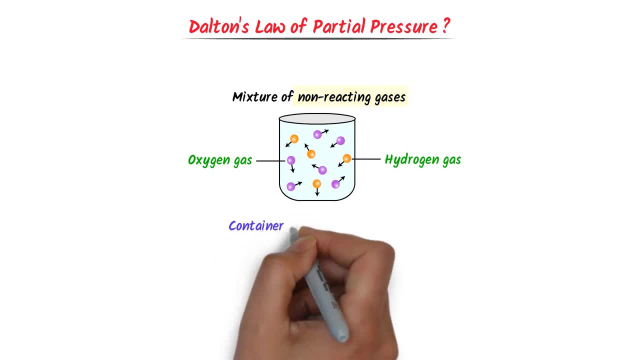 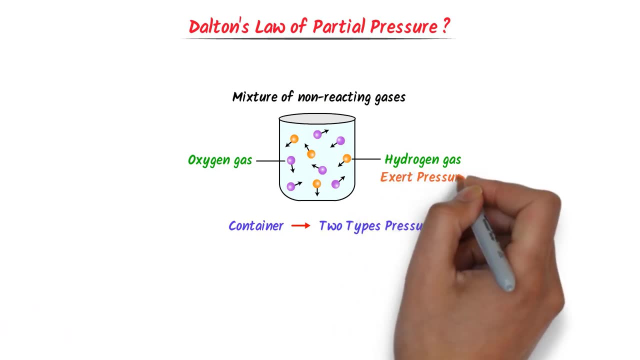 gas do not react with each other. Now this container experiences two types of pressure. I mean, the molecules of hydrogen gas exert pressure on the walls of the container. Secondly, the molecules of oxygen gas also exert pressure on the wall of the container. Now let me ask you: what is the total pressure on the wall of the container? The answer is simple. 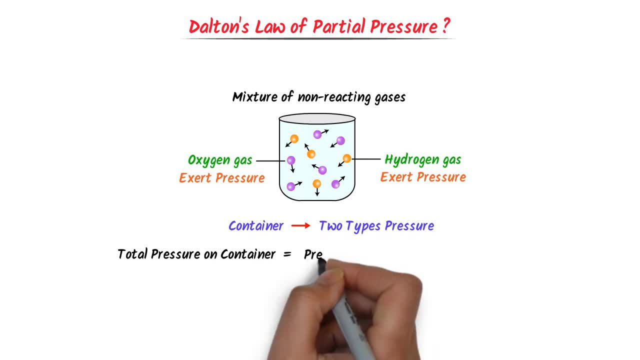 The total pressure on the walls of the container is equal to pressure of hydrogen gas plus pressure of oxygen gas. Are we right? total pressure Pt is equal to pressure of hydrogen gas plus pressure of oxygen gas. Therefore we define Dalton's law of partial pressure as: 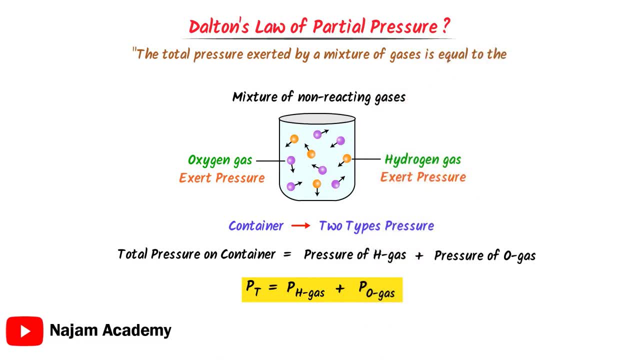 the total pressure exerted by the total pressure on the whole container. Victory exerted by a mixture of gases is equal to the sum of the partial pressures exerted by each individual gas. For example, let hydrogen gas exert 2 atmospheric pressure and oxygen. 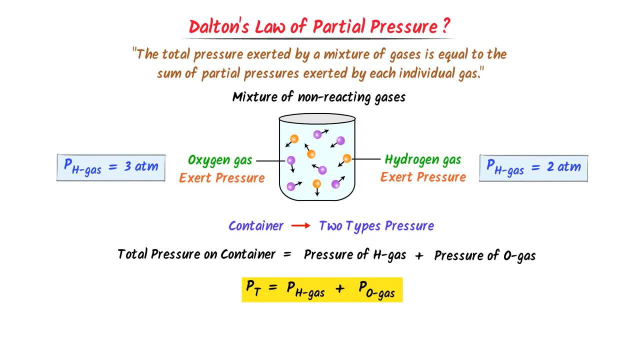 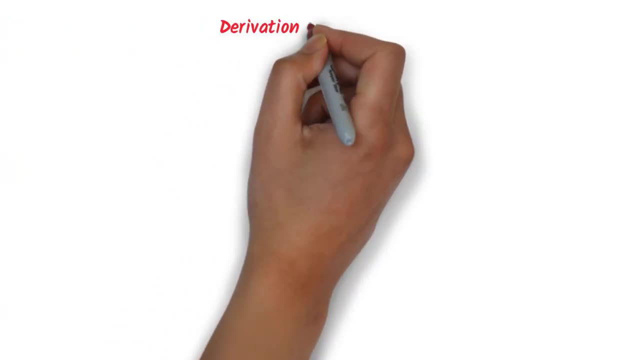 gas exert 3 atmospheric pressure, Then according to Dalton's law, the total pressure is equal to 2 plus 3 equals to 5 atmospheric pressure. Just note it down, all these important points. Now I will teach you the derivation of Dalton's law of partial pressure. Consider a mixture: 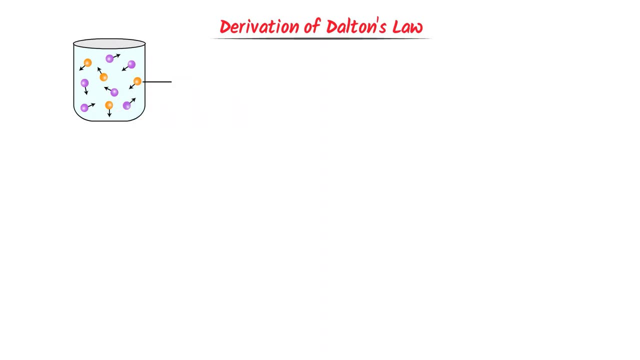 of non-reacting gases in this container. Let this is gas number 1 and this is gas number 2.. Now, according to ideal gas law, total pressure of these two gases, Ptn to V, is equal to 1 number of moles of first gas plus number of moles of second gas into Rt. Let this is. 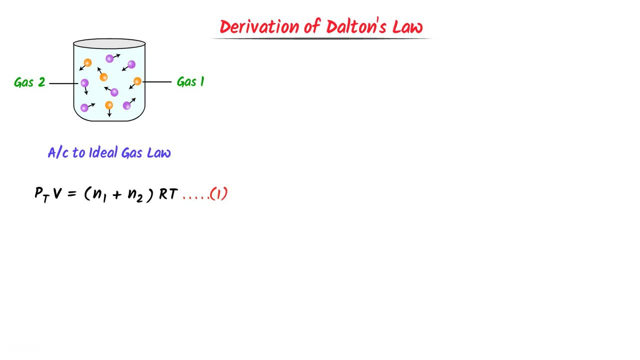 equation number 1.. Secondly, according to ideal gas law, the pressure of first gas on the wall of the container is: P1 into V, equals to number of moles of first gas into Rt Let. this is equation number 2.. Similarly we can also write the pressure of second gas. 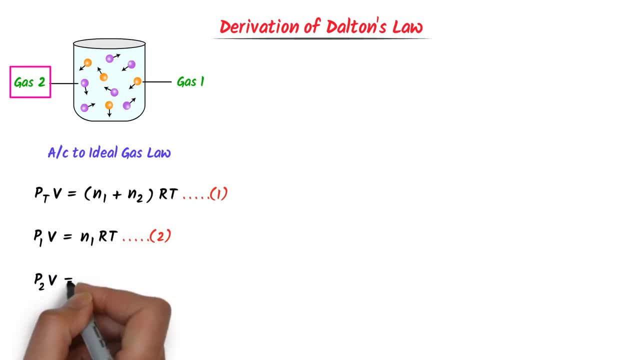 on the wall of the container is P2 into V equals to number of moles of second gas into Rt. Let. this is equation number 3.. Now listen carefully. I divide equation number 2 by equation number 1.. The equation number 2 is: 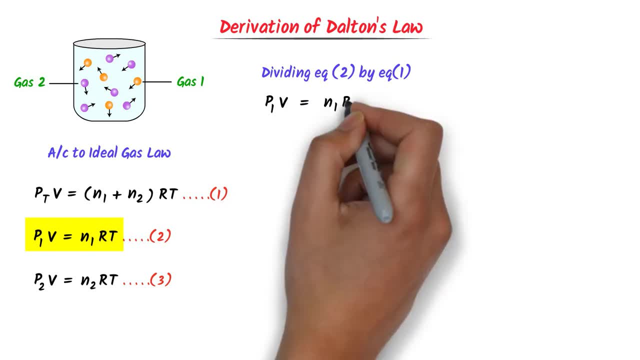 P1 V equals to N1 Rt upon the equation number 1 is Pt V equals to N1 plus N2 into Rt Here, this Rt and this Rt cancelled out This V and this V also cancelled out. We get: P1 upon Pt is equal to N1 upon N1 plus N2.. We know that mole fraction x is: 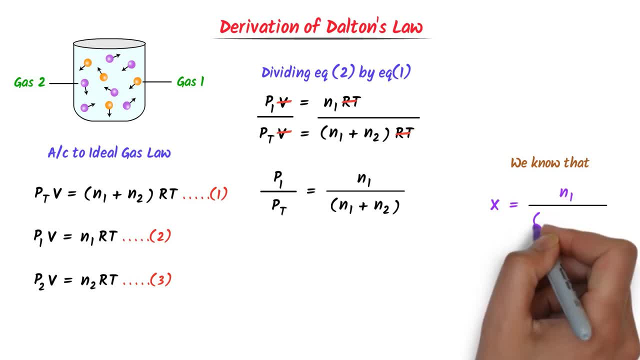 equal to number of moles of one specie upon total number of moles. Hence this thing is the mole fraction of first gas. I write P1 upon Pt is equal to x1.. I shift this Pt to the right-hand side. I get P1 is equal to x1 into Pt. It means that partial pressure. 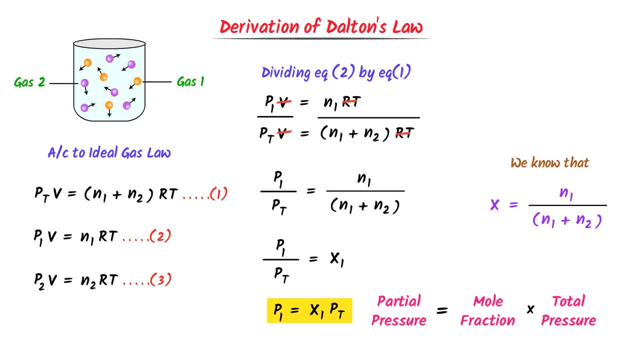 of first gas is equal to mole fraction of first gas into total pressure. If you want to learn more about mole fraction, watch our video and ask your questions in the comment section. It's link is given in the description. Secondly, I divide equation number 3 by equation. 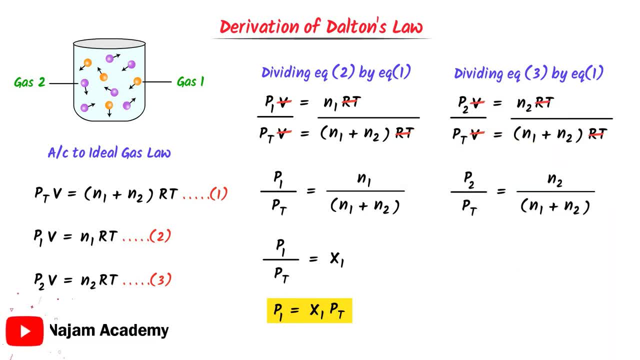 number 1.. After calculation I get: P2 is equal to x2 into Pt. It means that partial pressure of second gas is equal to mole fraction of second gas into total pressure. Thus this is the equation of Dalton's law of partial pressure. 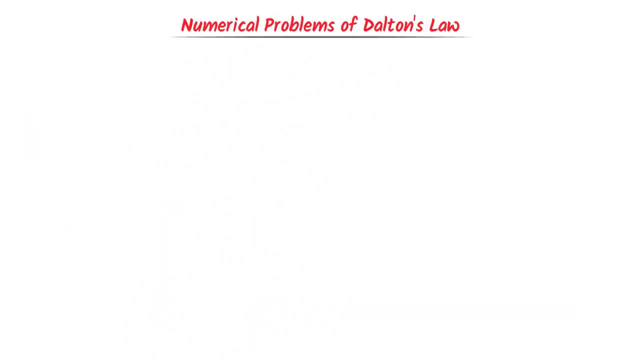 Now let me teach you important numeric equations. Consider this numerical problem of Dalton's law of partial pressure. A mixture of gases contain 4 gm of hydrogen gas and 32 gm of oxygen gas. Calculate the partial pressure of each gas. The given volume is 4 L and the temperature is 25 ºC. 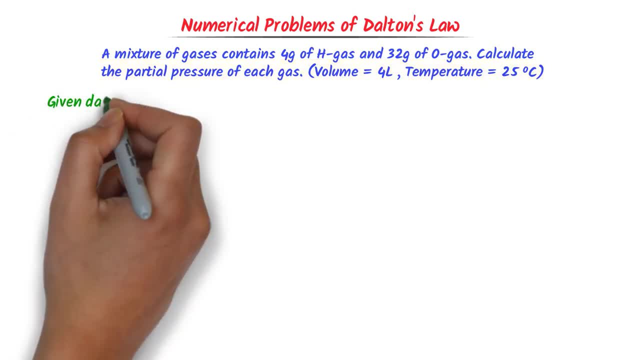 Now here is only one example of this example. First I write the given data: The given mass of hydrogen gas is 4 gm and the given volume of hydrogen gas is 12 gm. The given mass of oxygen gas is 13 gm. Then I write here: bar M 1, root: 2.. For the previous job in the 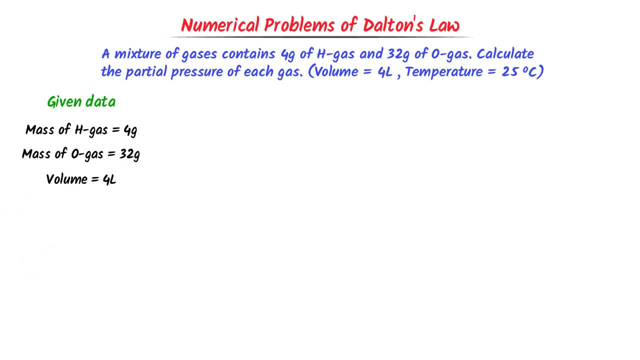 case is 32 g, the given volume is 4 L and the given temperature is 25 °C. I convert this temperature from °C to Kelvin. 25 plus 273 equals to 298 Kelvin. Here I write the value of R, Which is equal to 0.00821 l atm per mol. Now I calculate the number. 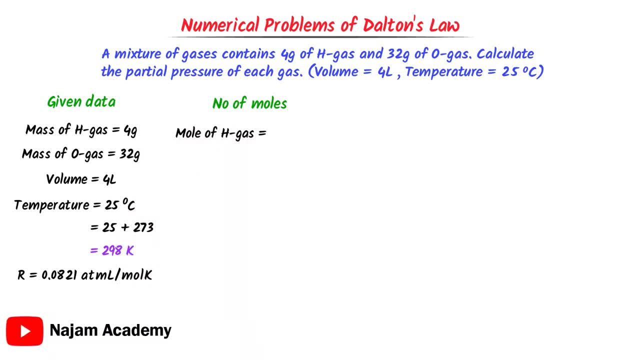 of moles of hydrogen gas, which is equal to given mass, which is 4 g, upon molar mass, which is 2 g per mole, I get 2 mol. Secondly, I calculate the number of moles of oxygen gas, which is equal to. 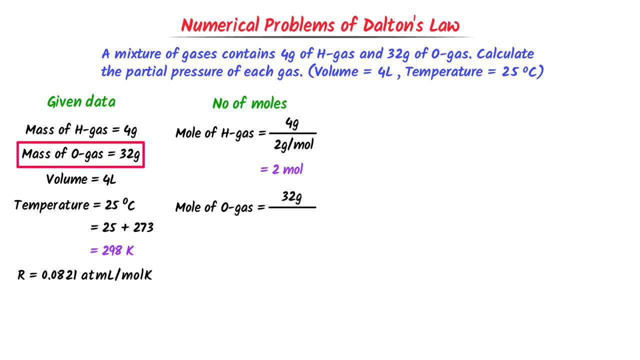 to given mass, and that is 32 g upon molar mass and that is 32 g per mole, I get 1 mole. Hence the number of moles of hydrogen gas is 2 mole and the number of moles of oxygen gas is 1 mole. Now I will calculate the total pressure According to ideal gas law: P total. 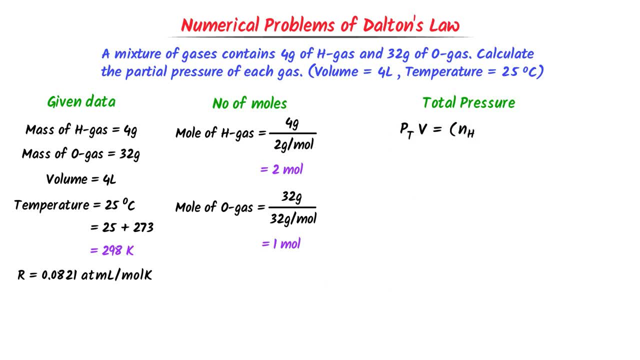 N2V is equal to number of moles of hydrogen gas plus number of moles of oxygen gas into RT. The given volume is 4.. Pt into 4 equals to the number of moles of hydrogen gas is 2 plus that of oxygen gas is 1.. The value of R is 0.0821 and 2. The given temperature. 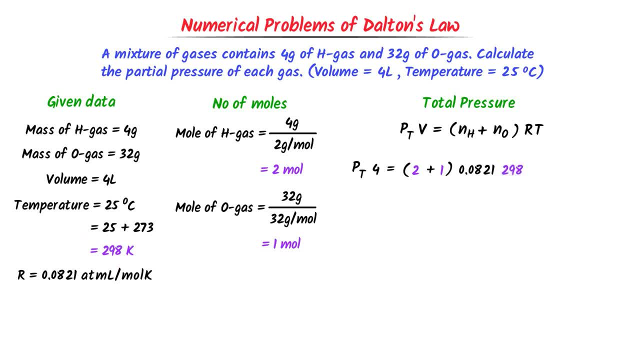 is 298 Kelvin. After calculation I get total pressure is equal to 18.349 atmosphere. Now I can easily calculate the partial pressure of hydrogen gas and oxygen gas. The partial pressure of hydrogen gas is equal to mole fraction of hydrogen gas into total pressure. Mole fraction is number. 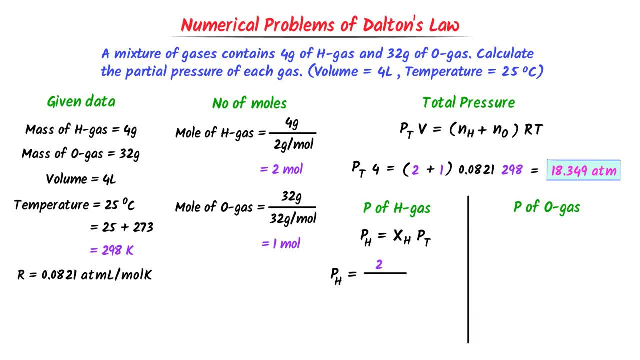 of moles of hydrogen gas, which is 2 mole, upon total number of moles, which is 1 mole, and the number of moles of oxygen gas is 2 moles. by 2 mole N2, total pressure is equal to 18.349 atmosphere, which is a drop ratio which measures 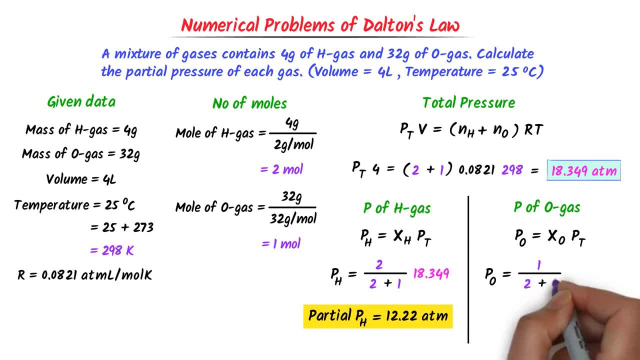 Your total pressure is equal to 18.349 atmosphere, which is a drop ratio which is up to12 atmosphere. 開э blankets. The number of the moles of oxygen gas is 1 per total number of moles of hydrogen gas. Pt is equal to mole fraction and K nickel, So this is 1.3 moles of lithium gas plus 2.4 moles are total moles of oxygen gas, which is 1 atom. 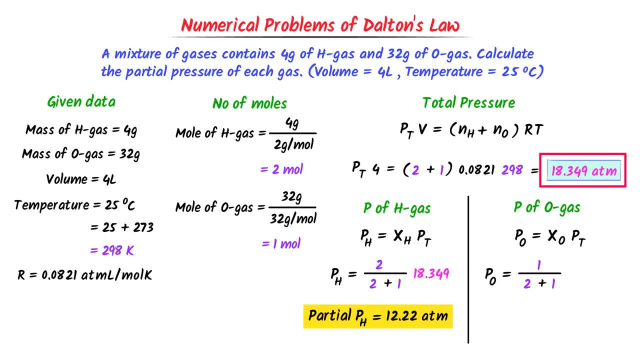 moles and to total pressure, which is 18.349.. After calculation I get 6.11 atmospheric pressure. Hence the partial pressure of hydrogen gas is 12.22 atmosphere and the partial pressure of oxygen gas is 6.11 atmosphere If we add the partial pressure of hydrogen gas and oxygen. 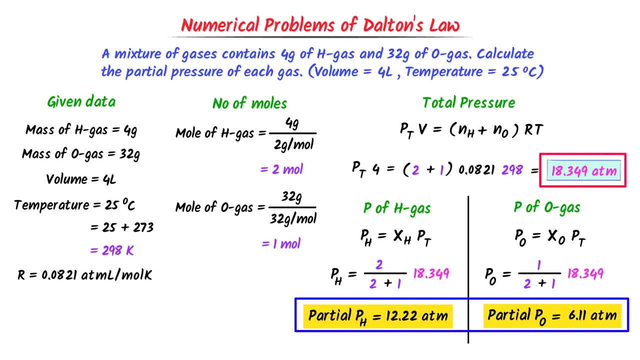 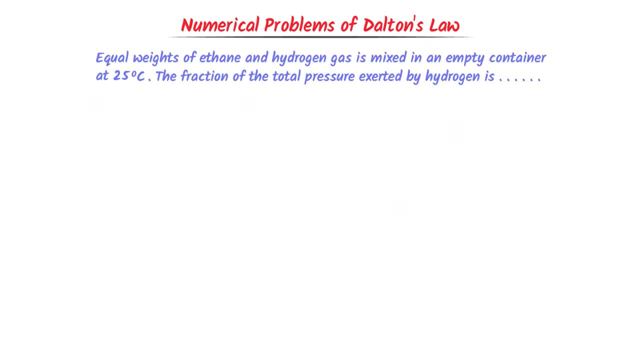 gas, we will get total pressure which is 18.349 atmosphere. Hence, noted down this important numerical problem. Lastly, let me teach you one important MCQs from competitive exam of IIT. Equal weights of ethane and hydrogen gas are mixed in an empty container at 25 degree centigrade.